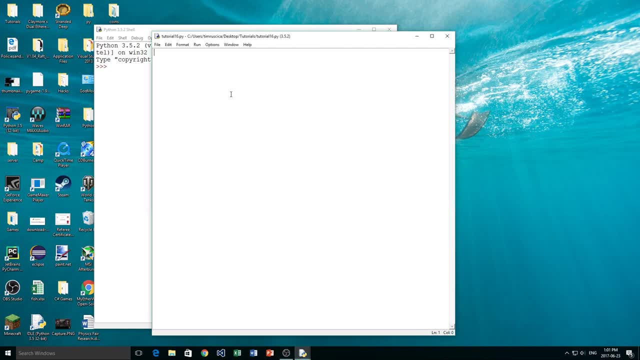 Hey guys, welcome back. This is the 16th video in my Python programming series, and today we're going to be talking about Python modules and import statements. So this is something new that I haven't talked about yet. but Python is a modular programming language, meaning that we can use multiple files together to create one program. 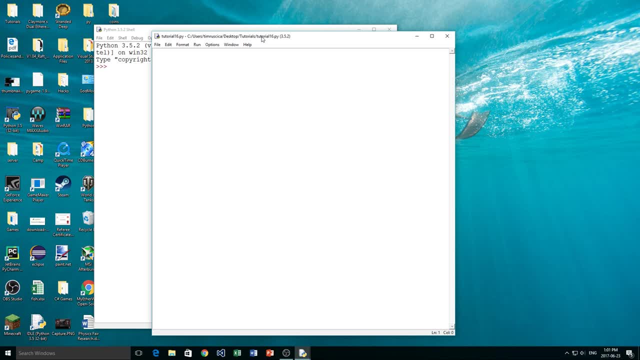 And you'll understand what I mean later in the video when I show some examples. But yeah, so pretty much in Python, at the beginning of all your Python scripts, what you typically do is you write something like this: It says import, and you can see this highlights an orangey-yellow meaning that it is a keyword in Python. 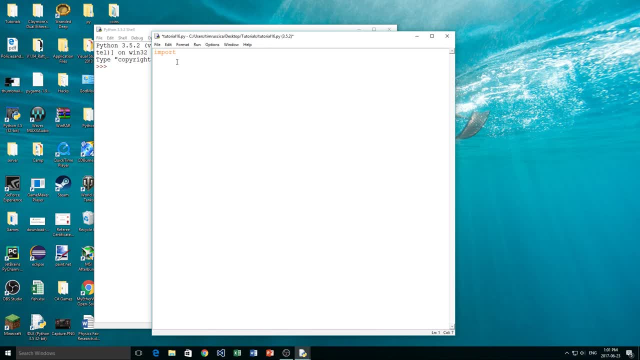 Now there are many built-in modules, or what they're called in Python, that contain a list of functions and classes that we can use in our Python script. So, for example, the math module import math. This allows me to do things like dot. 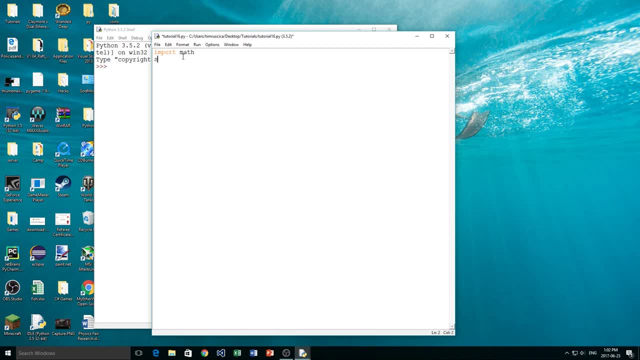 Square root or the square root function, which I believe is like this, And then you can put something inside of it. So yeah, there's plenty of cool things like that. There's another module. it's called PyGame. We're going to be doing this later. I'm going to be talking about game development with Python. 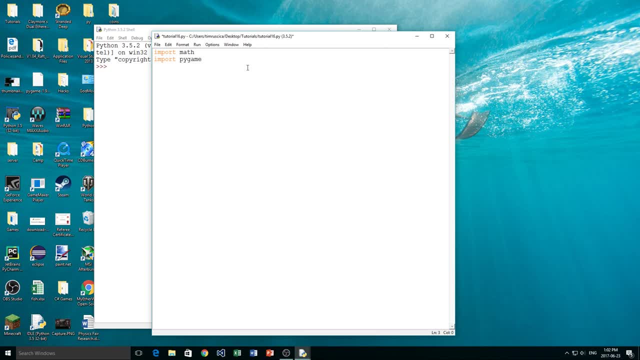 If you want to see that, leave a comment down below and I'll get it started soon. And then we have import. We can also import something called OS, And this gives us opportunity to do things like file And lots of different things like that. 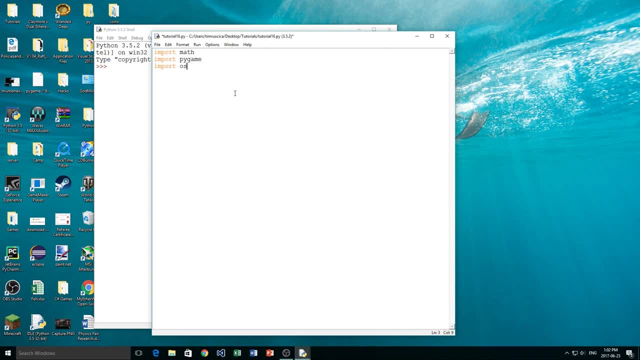 We can import images. we can import tons of different things into our files in Python. So we're just going to use the math module today for demonstration purposes. But pretty much what happens is there's a bunch of built-in modules in Python, So this one is known as a built-in module. 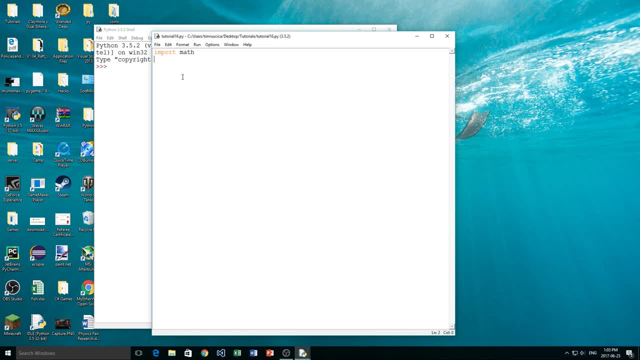 Math. when you download and install Python, it pretty much you download that module. The PyGame module that I was talking about is not a built-in module. That means you actually have to go to the internet. You have to find it and install it on your computer before you can import it into your Python program. 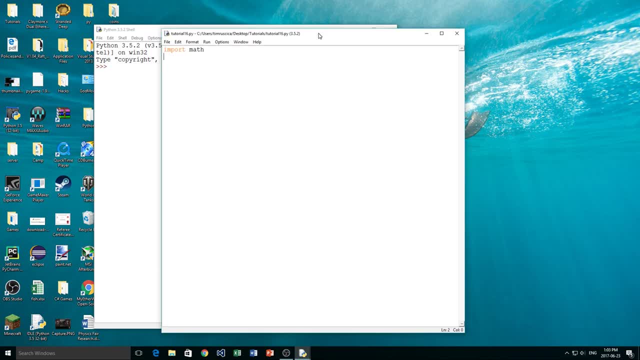 And now, what's really cool about Python is that it's an open-source language, Meaning that you can actually create your own modules, And they contain functions, classes, and you can use them in many of your different programs, Or you can also send them to a friend, maybe, or post them online for other people to be able to use. 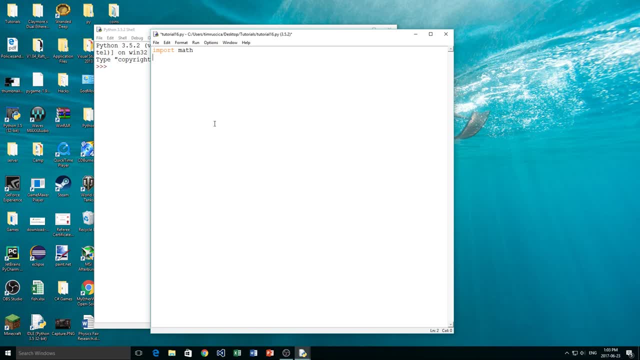 So let's get right into it and let's do some things here. So if we want to use this module, we're going to need to do a couple of things. So if we want to use this module, we're going to need to do a couple of things. 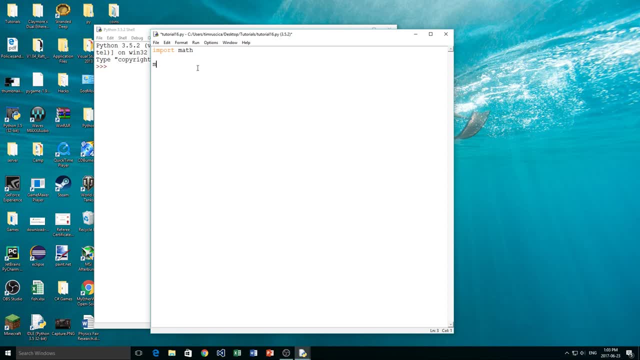 So if we want to use this module, we're going to need to do a couple of things. So if we want to use this math module, we have to first start by typing math, So the name of our module here, so math. 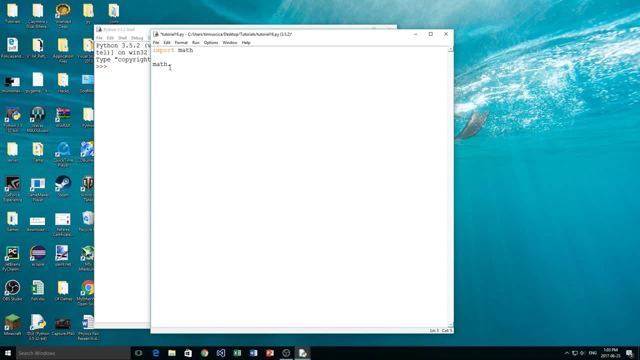 And then afterwards we're going to do the name of a function or a class in that math module. So you see a bunch of things pop up there in that little box. So if I do the dot again and wait a second, it should pop up. 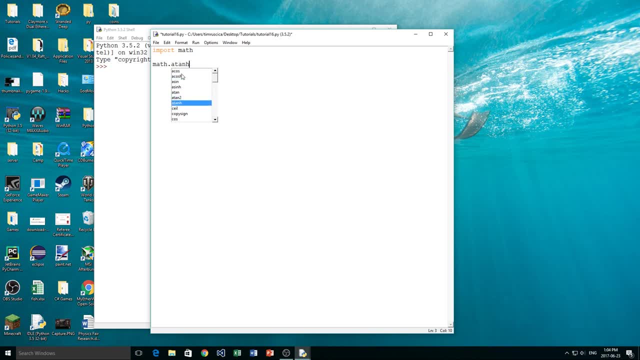 Yeah, so there we go, And you see we have cosine sine tangent, all that stuff, degrees, factorial, all these things Inside of our math module. So these are new things that we wouldn't be able to use before. 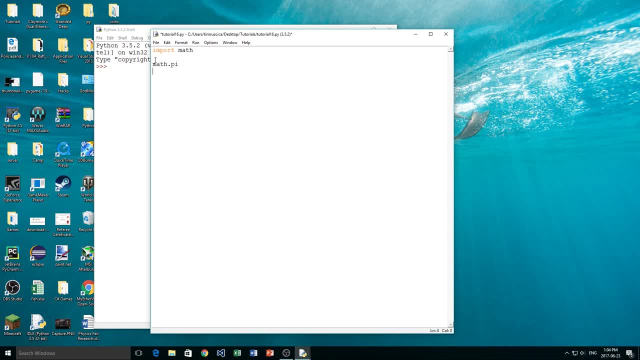 So I'll show you, if we do mathpy and I print that to the screen, well, we should get an endless number of digits like this: mathpy, Is it running? There we go. So I just had to print a bunch of numbers. 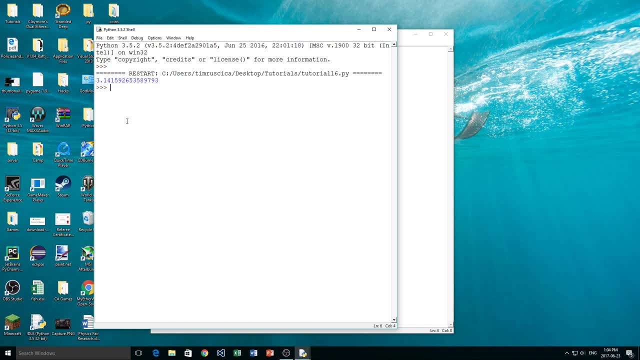 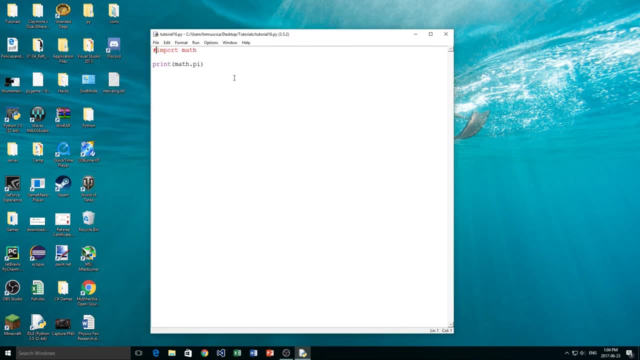 So mathpy, it didn't print all of them. I think it only went to 10 decimal points. So yeah, and then I'll show you, if I comment out this import math, what will happen if I try to do this: We get an error because, well, math is not defined. 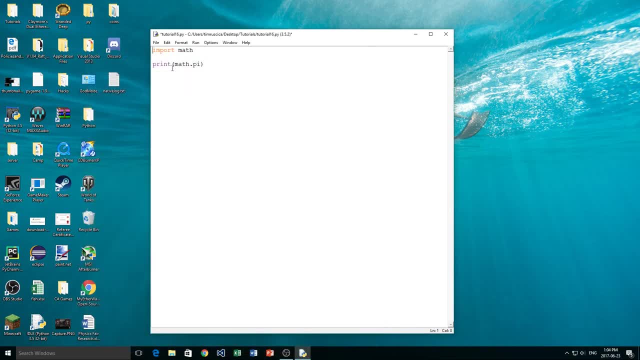 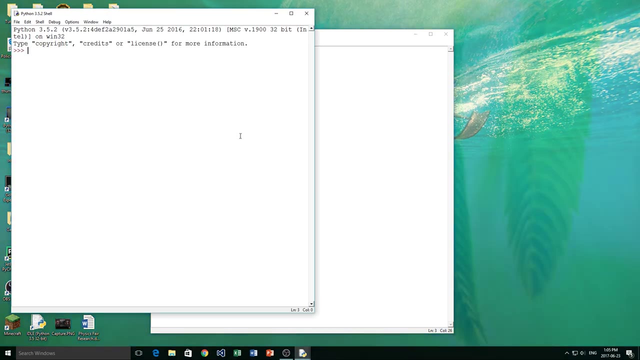 We didn't import it at the top of our program, So we'll uncomment this now. Now I can do things like mathdegrees. Degrees simply turns something that is in radians into degrees. So if I did mathpy in here, for example, and we print that to the screen, we get 180. 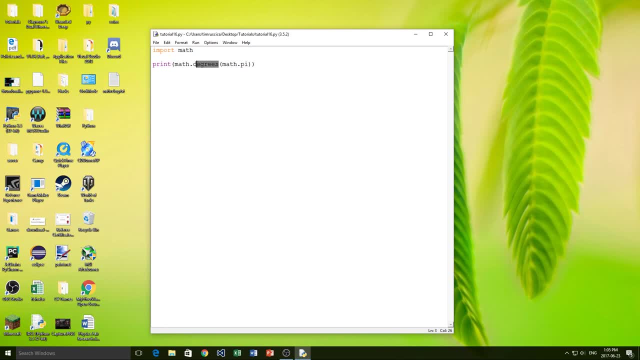 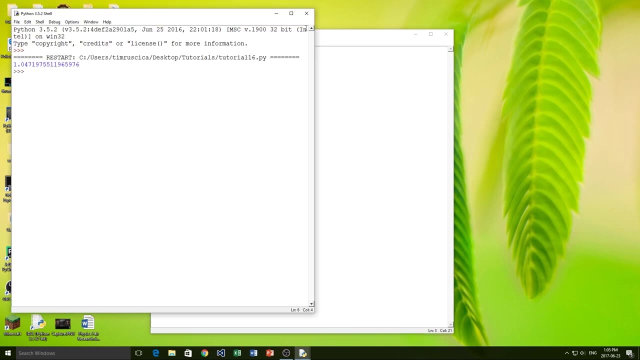 degrees like that, They also have the mathradians, I believe, which does the opposite, So it turns a degree into a radian. So if we did 60 degrees here like that and we get 1.047, which is about pi over 3 radians. 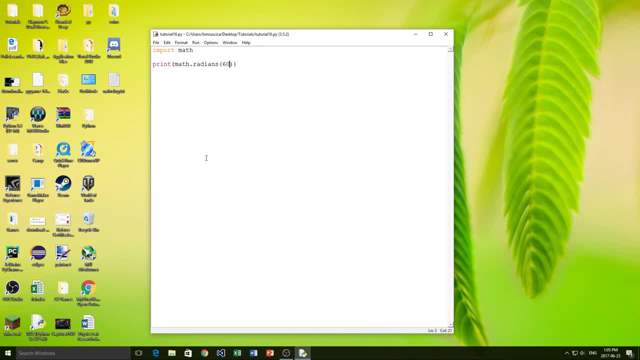 like that. So, yeah, there's lots of cool things that we can do with these modules. Now I'll actually show you an example of how we can use our own modules and how we can import our own modules into our function. So I'm going to just start by typing import and I'm going to type mymodules. 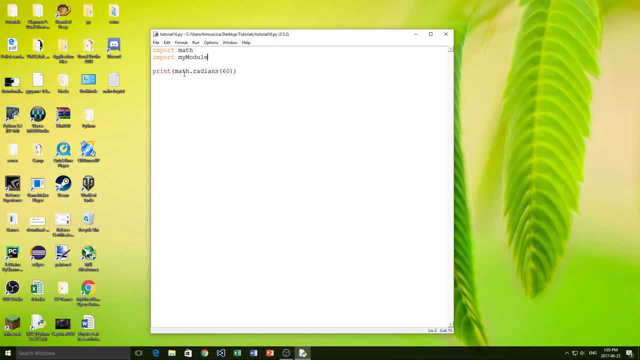 Now I haven't actually created this module yet. We're going to do that in just a second. Now I'm going to go and I'm going to find the directory that my main script is in, So it's in tutorials up here. I've got this open and remember how we had the file in here as well, because it has to. 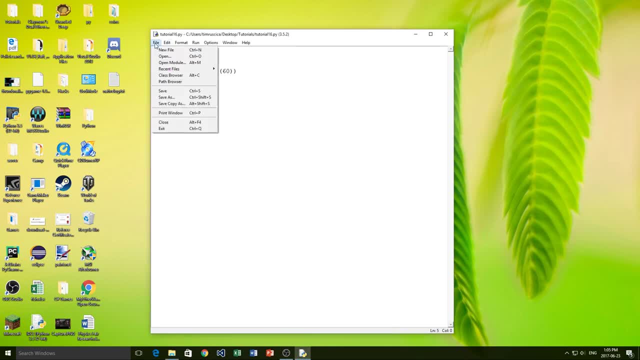 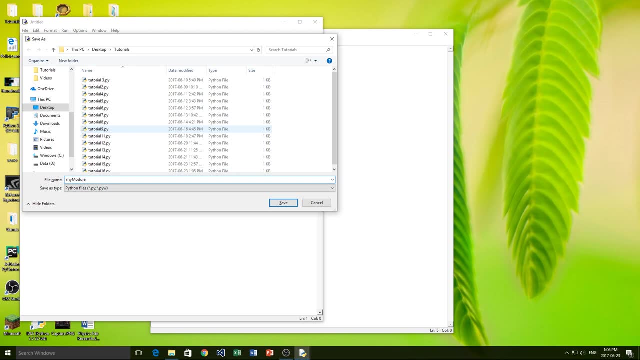 be in the same directory. So I'm going to create a new file in that directory. So file new file. I'm going to save this one as mymodule. Now, spelling is very important- Again, capitals do matter- And it has to be in the same directory. 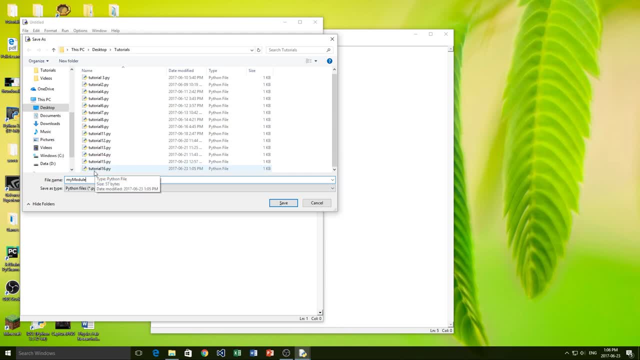 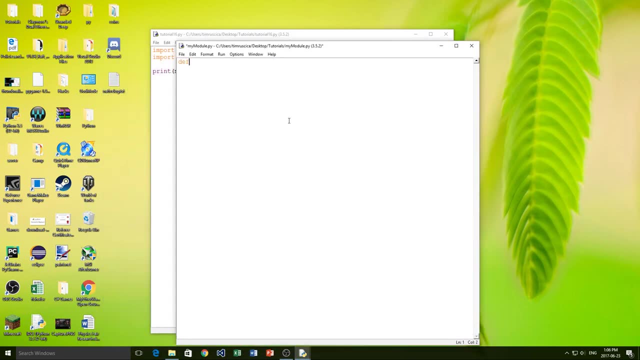 And it has to be in the same directory as our main script, which it is like that. Now, inside of this module, I'm going to write a very basic function. If you haven't seen that video yet, go check that out first. 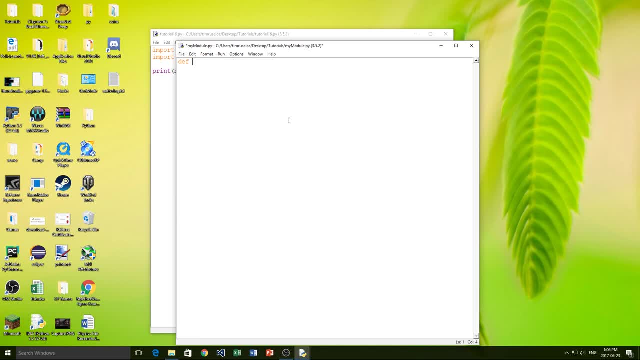 We just talked about some basic functions and what they do and the use of them. So I'm going to define- I'm just going to call it myfunc like this: It's going to take a parameter called x and all it's going to do is return x plus 5.. 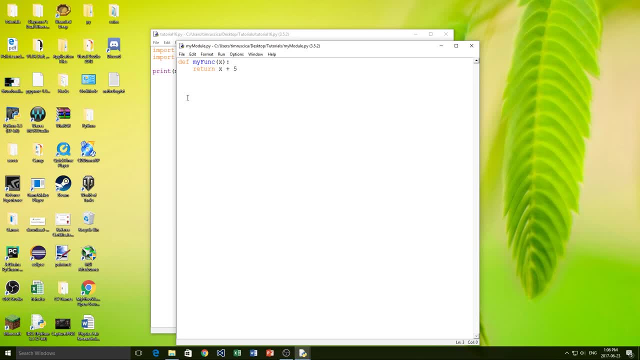 So very basic function like that, But just for demonstration purposes here. okay, And now I have mymodule imported like this, So I can actually use mymodule. So I'm going to do print mymodulemyfunc, because that's the name of my function. 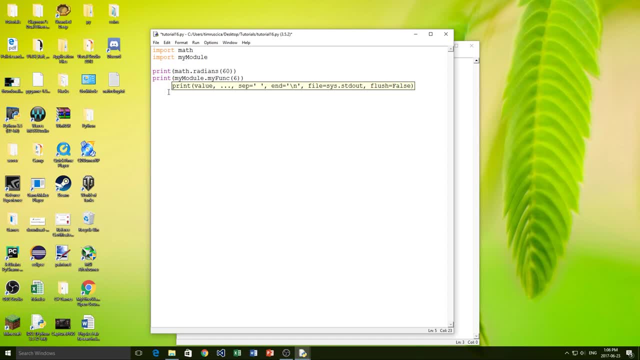 And then inside I need to give it a number. So what number do we want to use? Maybe we'll use 6. And we print this out And you see we get 11.. So, by simply, all I did was create a new file. 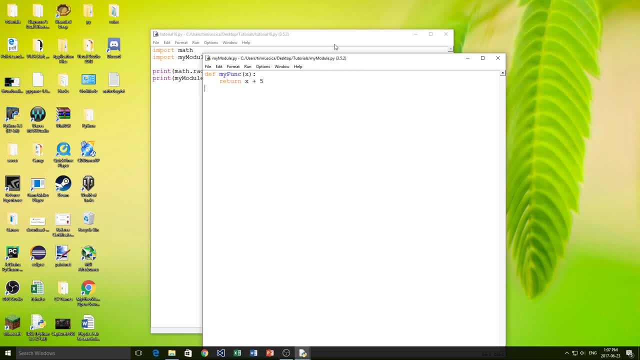 Put it inside of my Same directory as this script here And, easy enough, we were able to use it. Now I can actually create multiple functions in here, So I can create define another func like this: that'll be the name. This one will take x again. 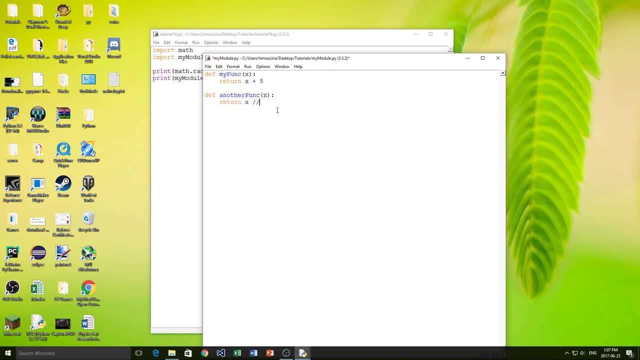 And inside here I'm going to return x, integer, division 5.. And then again we could use that one. So instead of myfunc we'll use another func like this, And let's just type in a big number like that and see what we get. 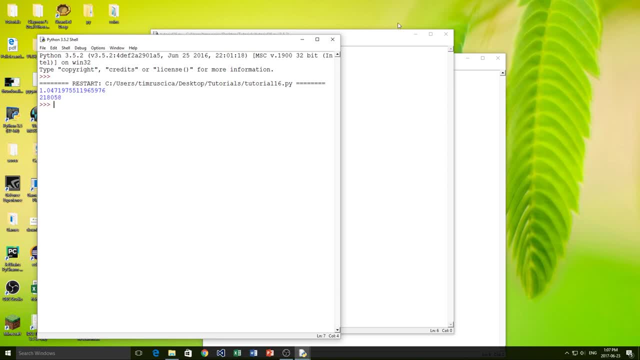 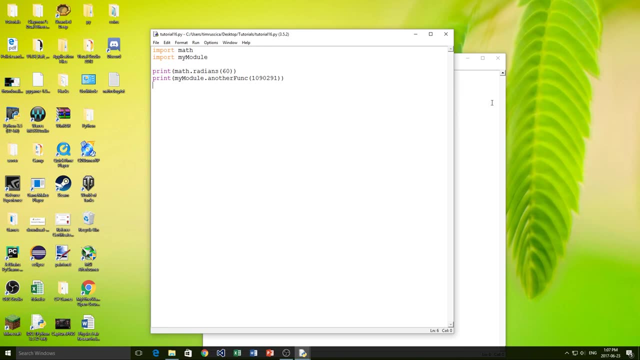 There we go, So again, it's working perfectly fine. So that's how modular programming- is what it's called- works in Python. Now, obviously, if you're going to be doing modular programming, it's usually for larger programs and bigger programs where you want multiple files to keep things organized.